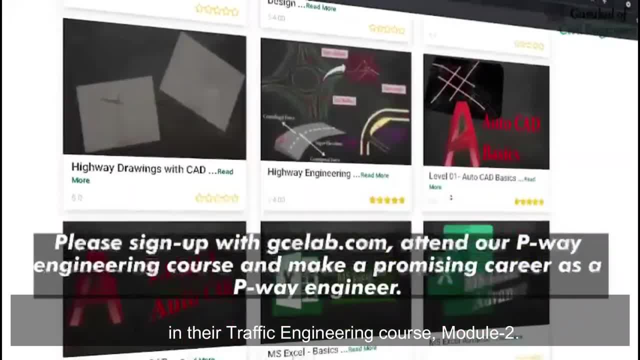 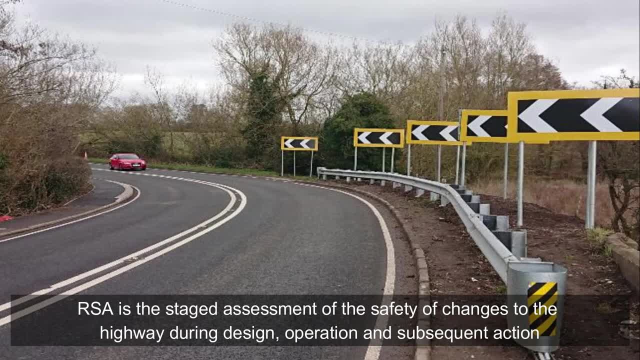 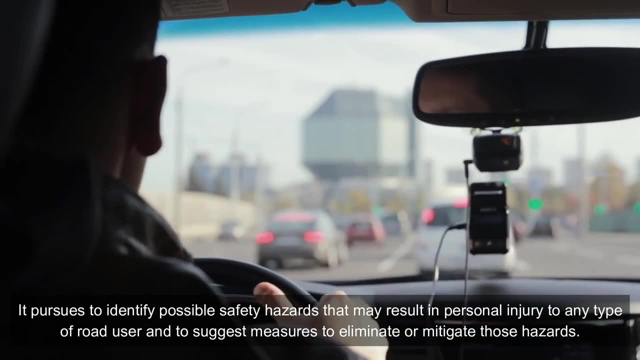 overview of road safety audit in their traffic engineering and traffic engineering courses. What is a Road Safety Audit? RSAT is the staged assessment of the safety of changes to the highway during design, operation and subsequent action. It pursues to identify possible safety hazards that may result in personal injury to any type of road user. 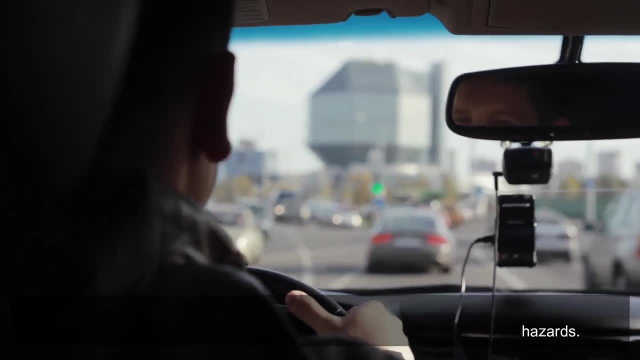 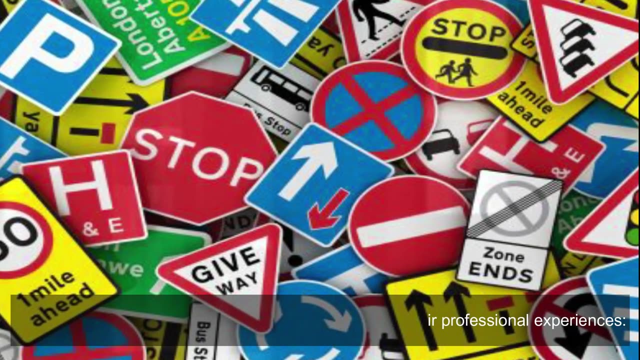 and to suggest measures to eliminate or mitigate those hazards. Type of road safety auditors: There are three levels of road safety auditors as per their professional experiences: 2. Road Safety Audit- Árbitresрасf, Cross- Bordersegment台, Bratislavabank. 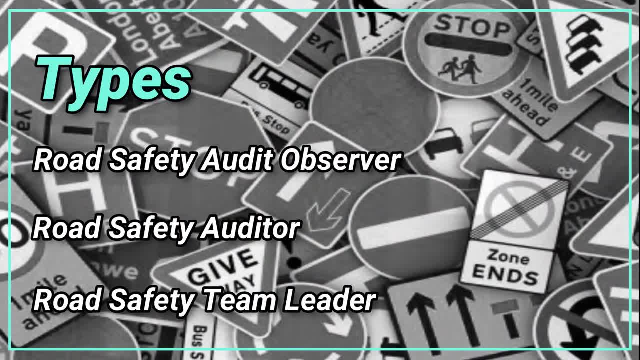 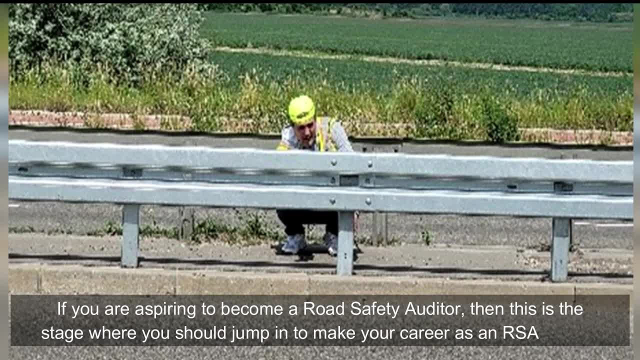 Group 얘기áoperação: Investigation of emails based on travel bookingáRSABáóa Road Safety Audit Observer. Road Safety Auditor, Road Safety Team Leader. Road Safety Audit Observer: If you are aspiring to become a Road Safety Auditor, 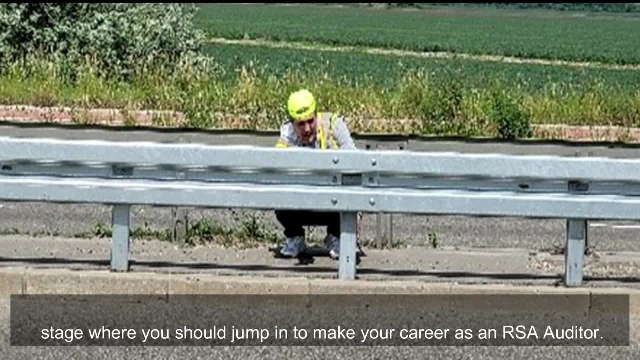 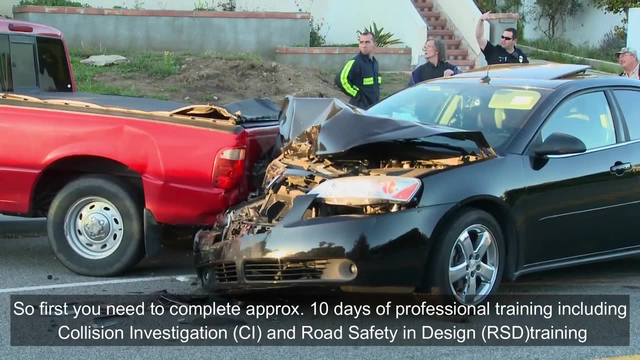 then this is the stage where you should jump in to make your career as an RSAL Auditor. So first you need to complete a PROCS: 10 days of professional training, including Collision Investigation, CI and Road Safety and Design. RSD Training- Road Safety Auditor. 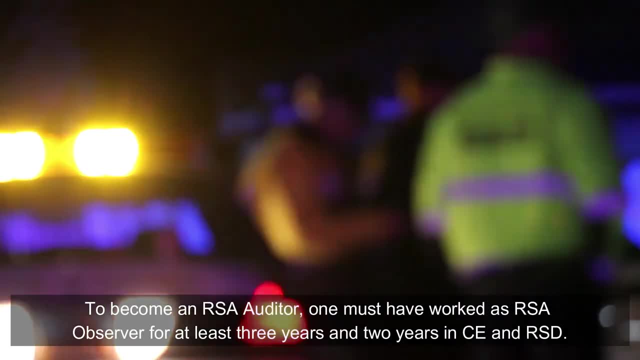 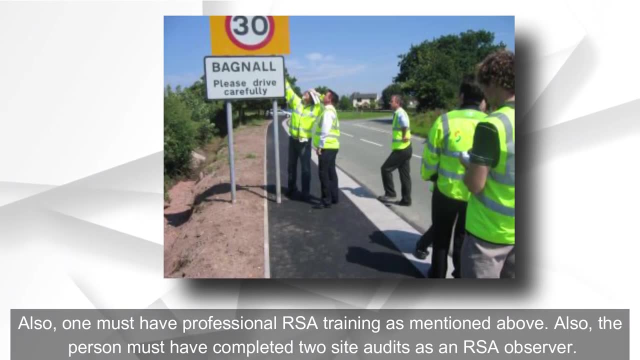 To become an RSAL Auditor one must have worked as RSAL Observer for at least 3 years and 2 years in CE and RSD. Also one must have professional RSAL Training, as mentioned above. Also, the person must have completed 2 site audits as an RSAL Observer. 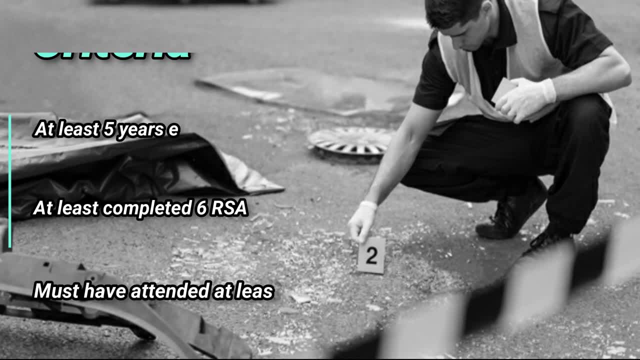 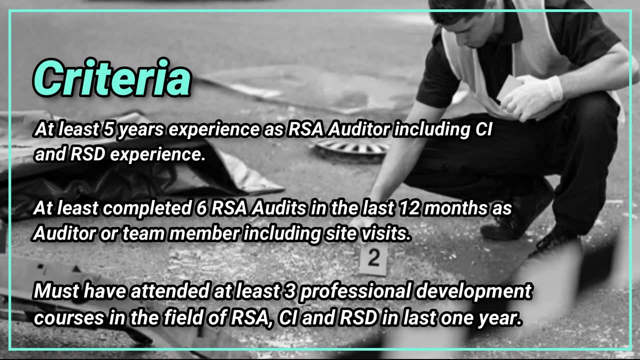 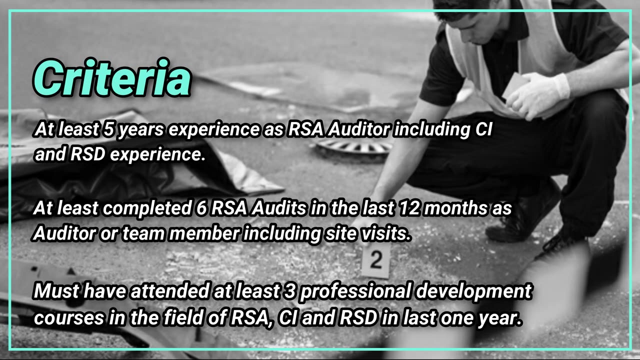 Road Safety Team Leader. Following are the key criteria to become an RSAL Team Leader: At least 5 years experience as RSAL Auditor, including CIA and RSD experience. At least completed 6. 6 RSAL Audits in the last 12 months as auditor or team member, including site visits. 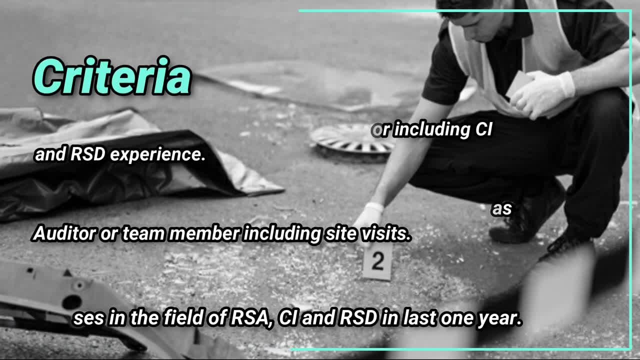 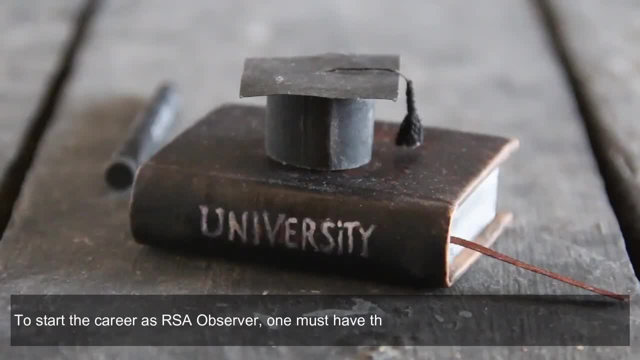 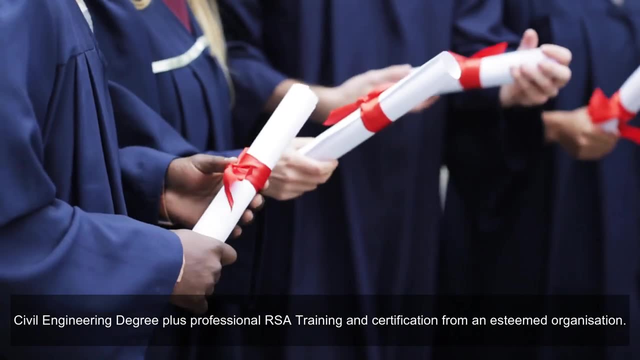 Must have attended at least 3 professional development courses in the field of RSAL, CI and RSD in last 1 year. Road Safety Auditor's Qualification: To start the career as RSAL Observer one must have the following professional qualification: Civil Engineering Degree plus Professional RSAL Training and Certification from an esteemed organization. 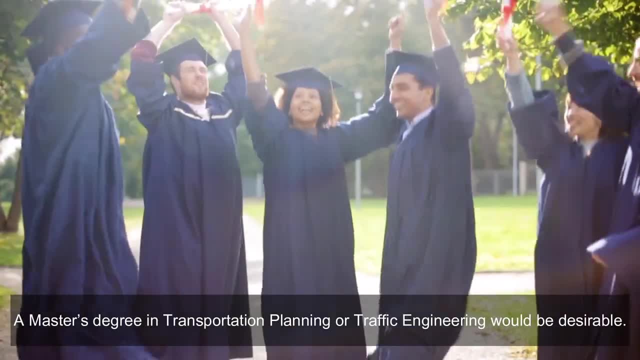 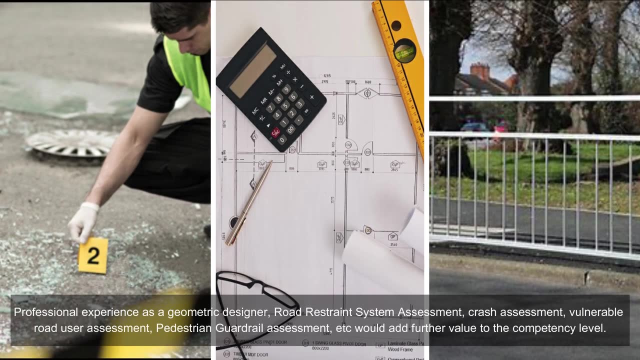 A Master's Degree in Transportation Planning or Transportation. A Master's Degree in Traffic Engineering would be desirable. Professional Experience as a Geometric Designer: Road Restraint System Assessment, Crash Assessment, Vulnerable Road User Assessment, Pedestrian Guardrail Assessment, etc. 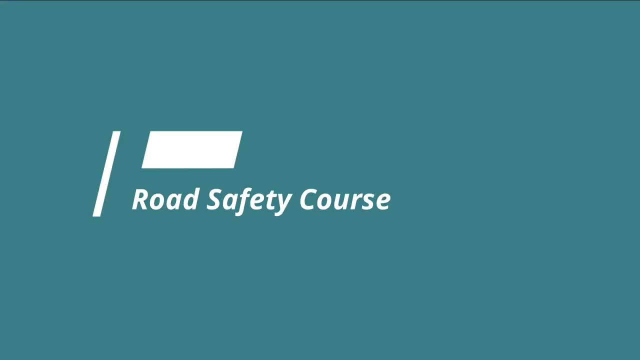 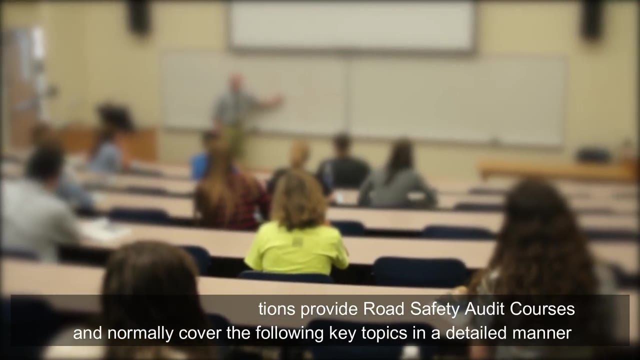 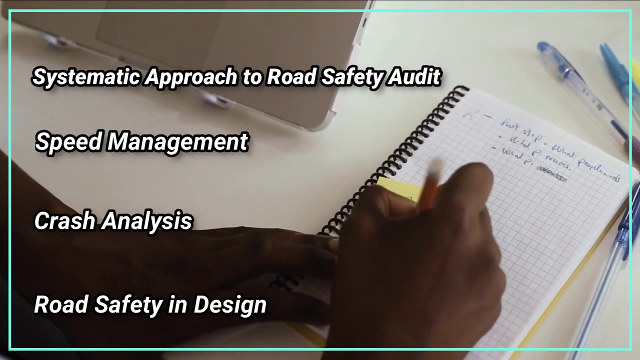 would add further value to the competency level. Road Safety Courses. Many professional institutions provide Road Safety Audit courses and normally cover the following key topics in a detailed manner: Systematic Approach to Road Safety Audit, Speed Management, Crash Analysis, Road Safety and Design. 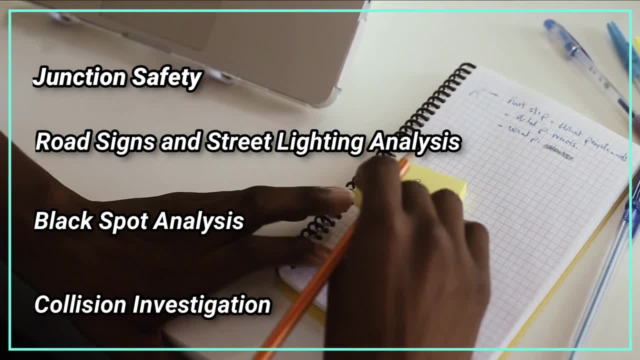 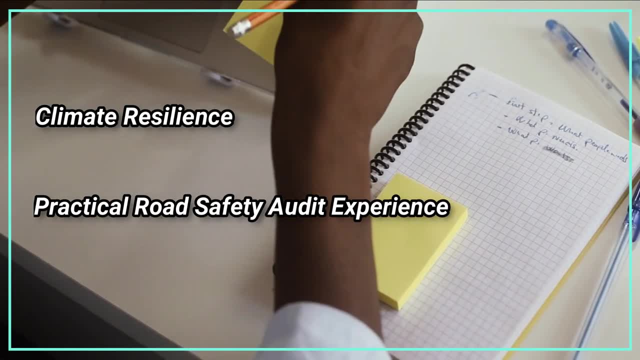 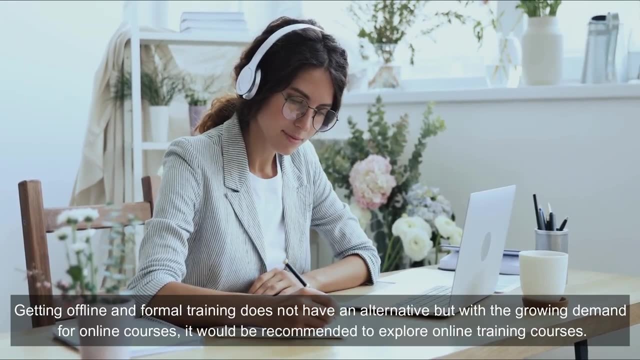 Junction Safety, Road Signs and Street Lighting Analysis, Black Spot Analysis, Collision Investigation, Climate Resilience, Practical Road Safety Audit Experience. Getting offline and formal training does not have an alternative, but with the growing demand for online courses, it would be recommended to explore online training courses. 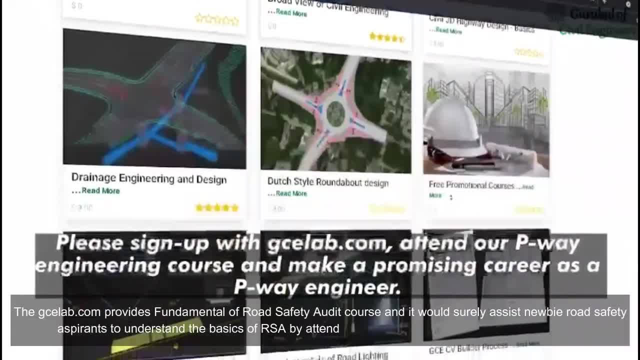 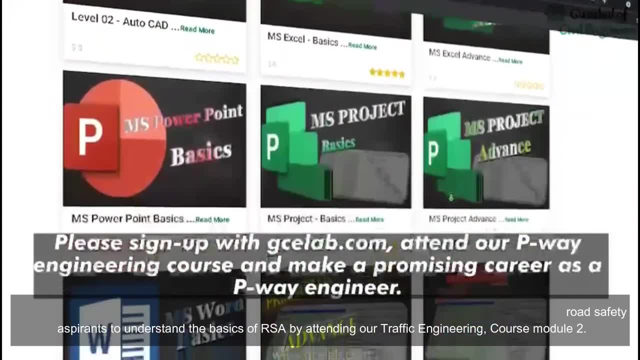 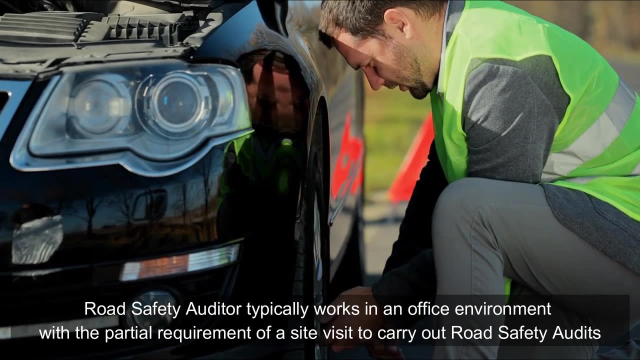 The gclabcom provides fundamental of Road Safety Audit course and it would surely assist Newbie Road Safety Aspirants to understand the basics of RSA by attending our Traffic Engineering Course, Module 2.. Road Safety Auditor Job. Road Safety Auditor typically works in an office environment with the partial requirement of a site visit to carry out Road Safety Audits. 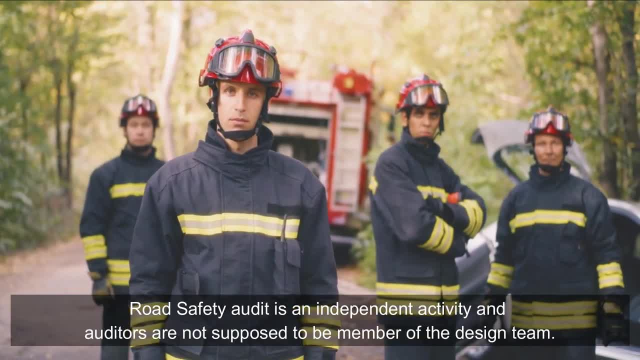 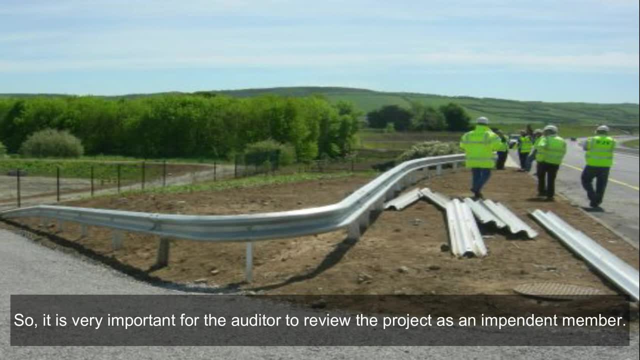 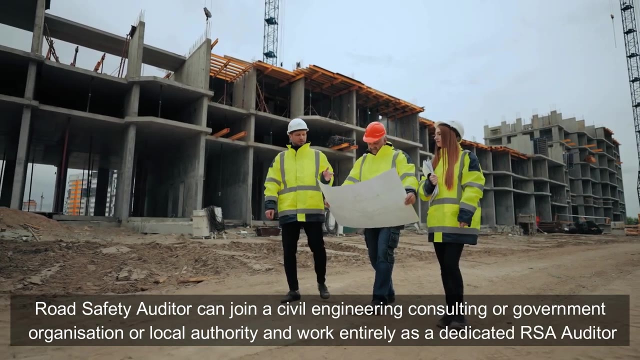 Road Safety Audit is an independent activity and auditors are not supposed to be member of the design team, So it is very important for the auditor to review the project. as an independent activity, Road Safety Auditor can join a civil engineering, consulting or government organization or local authority and work entirely as a dedicated RSA auditor. What is the average salary of Road Safety Auditors? The average salary for an entry-level road safety observer in the USA is around $67,000.. Although it varies from metropolises to small cities and competency levels, etc. The Road Safety Auditor role is very important. 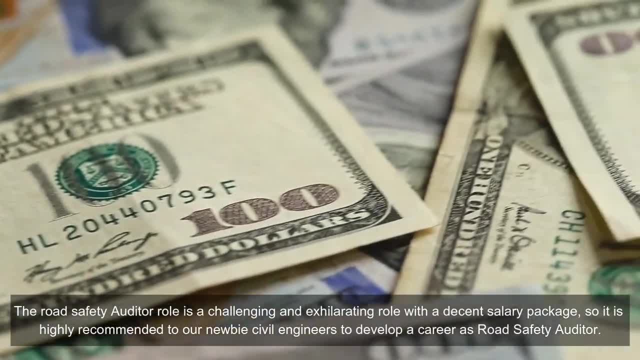 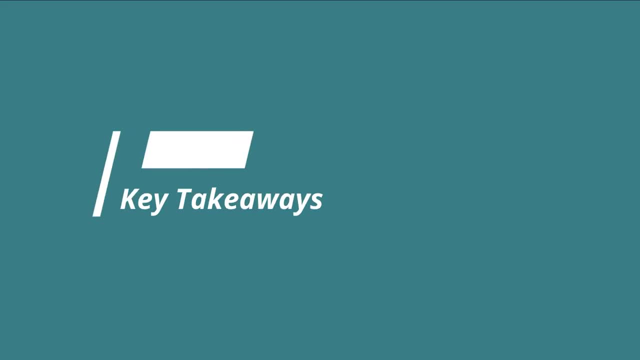 The role is a challenging and exhilarating role with a decent salary package, So it is highly recommended to our newbie civil engineers to develop a career as Road Safety Auditor. Key Takeaways: Road Safety Audit is a critical skill and in huge demand globally. 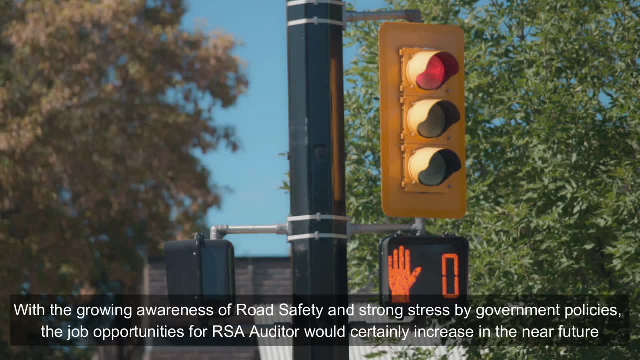 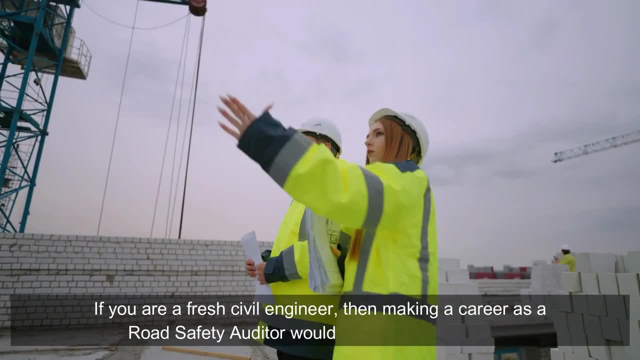 With the growing awareness of road safety and strong stress by government policies, the job opportunities for RSA auditor would certainly increase in the near future. If you are a fresh civil engineer, then making a career as a Road Safety Auditor would be a great opportunity. 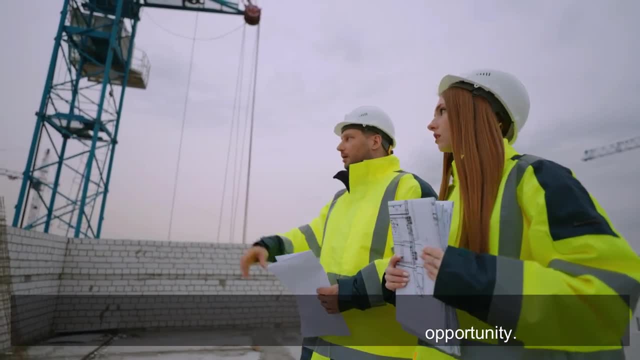 If you are a fresh civil engineer, then making a career as a Road Safety Auditor would be a great opportunity. I hope this video provides you with great understanding of how to become a Road Safety Auditor. I hope this video provides you with great understanding of how to become a Road Safety Auditor. 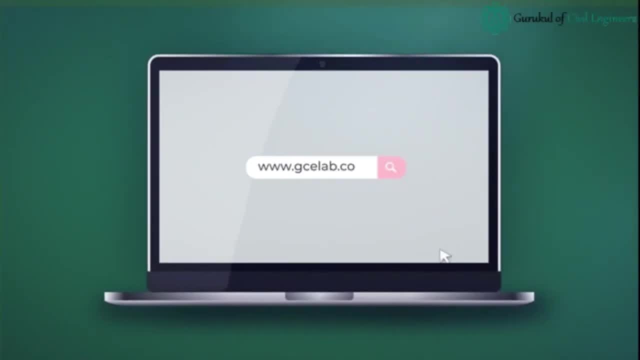 Please feel free to like, share and comment. Please feel free to like, share and comment.